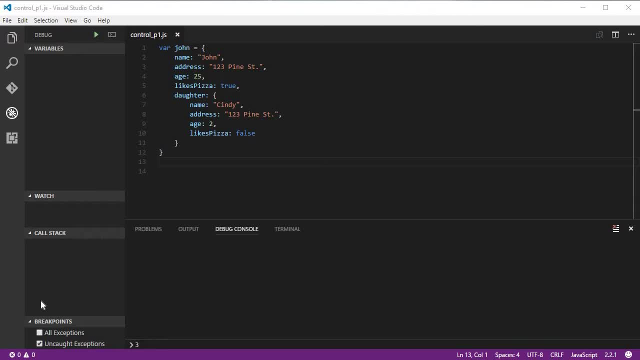 It just gives rise to, if else statements, logic statements. In other videos we'll be talking about switch statements and different types of methods of how to use logic, So let's get into it. So I took the variable John with his daughter, Cindy, and I just put it into one object like this so that we can do some tests on it. 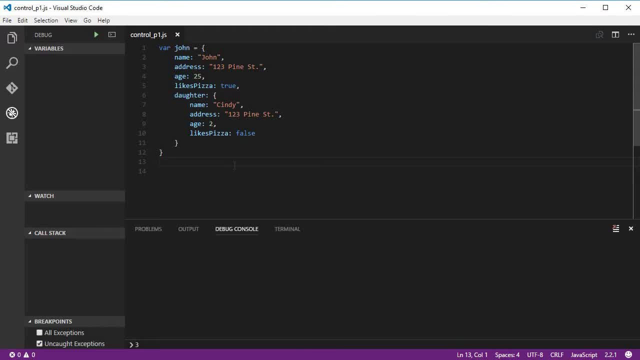 So the first thing we're going to do is we want to find out whether or not the whole family likes pizza. So how would we do that? So let's look at an if statement. So we're just going to say if. So, when we think about the family, we want to make sure that John and his daughter, Cindy, both like pizza. 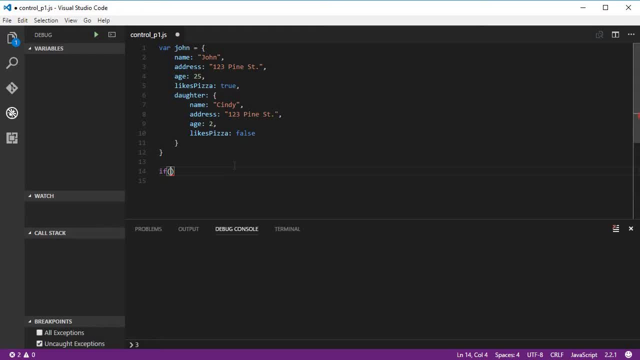 So that word and and is a logical operator. It means that both conditions will be true. So let's look at John likes pizza And is symbolized by these two ampersands. And then we're also going to say John daughter dot likes pizza. 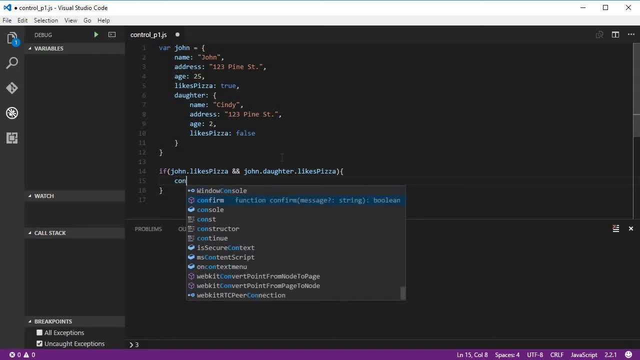 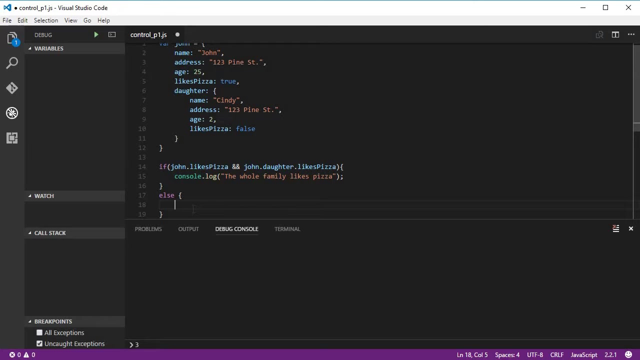 And if this is true, we're going to console log out. the whole family likes pizza. And then we're going to say else, And so else is going to say: if this is not true, then run this code. And we're going to say: someone doesn't like pizza. 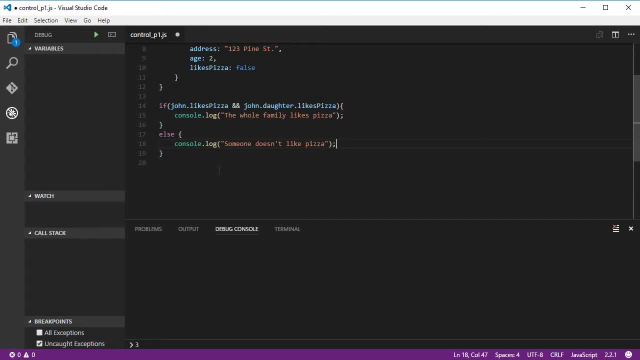 So normally in our code so far we've been doing ones that run top down. In this case we're going to control the flow of our code By testing whether or not it's true, By testing whether or not John likes pizza and his daughter likes pizza. 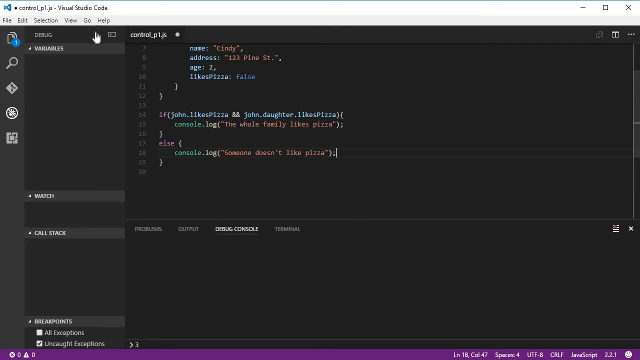 So let's figure out which one gets printed. Alright, so it skipped this line because John likes pizza but his daughter doesn't. So this would be false, So we go into this else statement. So what if we want to be a little bit more detailed and exact about who doesn't like the pizza? 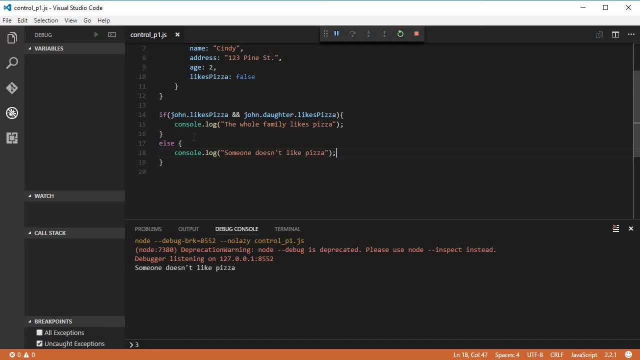 So this is where an if else statement comes in handy. So let's just modify this a little bit. So, instead of saying if this, then do this, If this is false, then do this, We're going to say: if this is false, then check again. another statement. 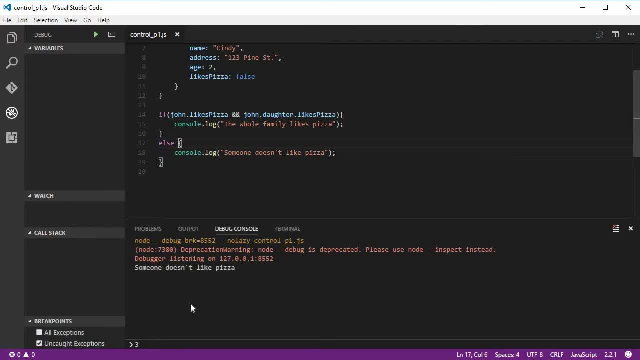 So that would be an if else. if So, we're going to say in here: if John likes pizza, Then we're going to say John likes pizza. Next check we're going to do is else. if So, what we're saying is: if both of them like pizza, no, 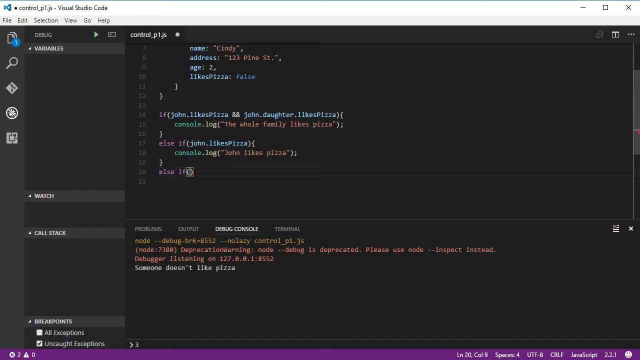 So does John like pizza? Maybe? If that doesn't work, then we're going to say: oh okay, let's try another one. Let's just see if John's daughter likes pizza, Cindy likes pizza, And in the last one we're going to say else. 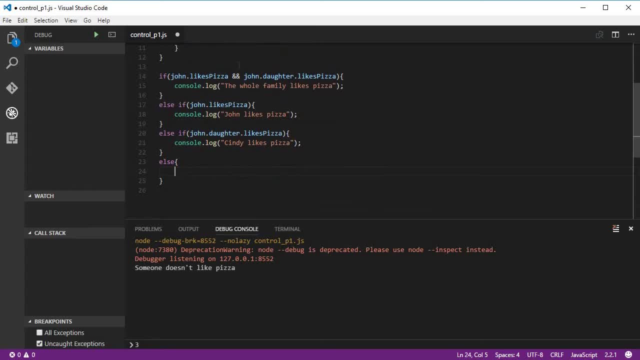 Else is just going to catch the last statement. If all of these fail, then we're going to say: no one likes pizza, So let's test this out. So the first one: we know that John likes the pizza, So let's just make sure that works. 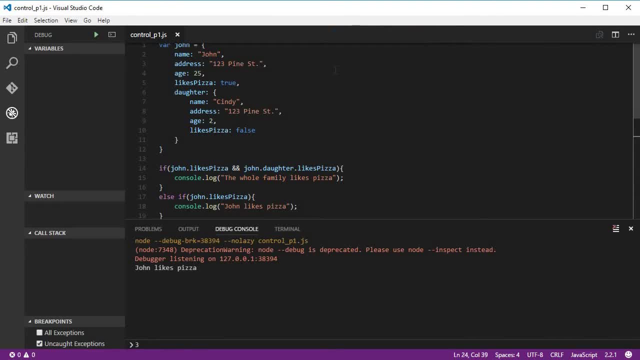 John likes pizza, All right, so how can we change this? So let's try saying that Cindy likes the pizza also When we run. we'll say: the whole family likes pizza. That's because both John and his daughter like the pizza. 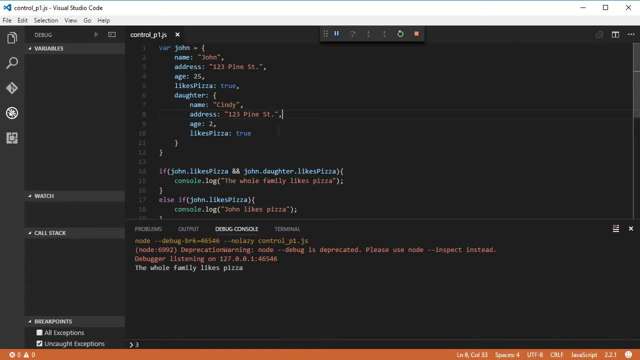 So let's try changing this. now Let's see that John doesn't like pizza, but Cindy does. In that case, Cindy likes the pizza. So how can we get no one likes the pizza? Well, if you guessed it, it's just as easy as just saying: you know, no one likes pizza. 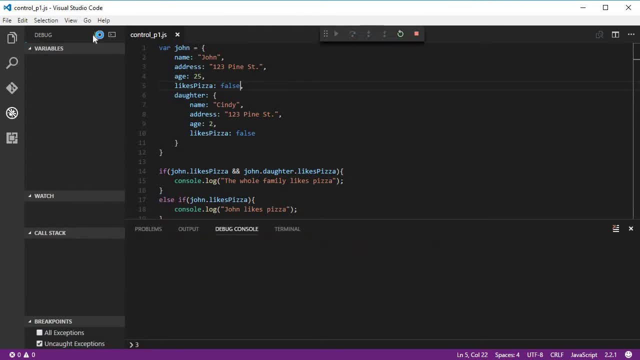 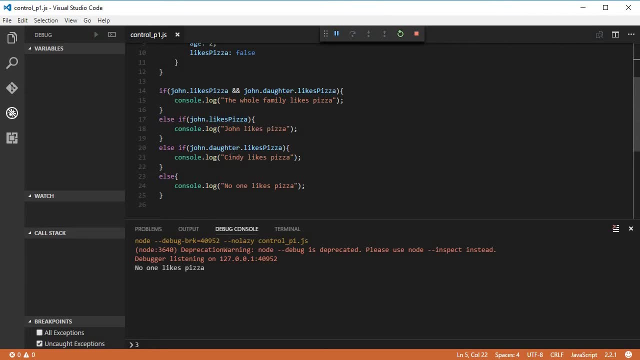 Just making sure that they both don't like pizza. Yep, and sure enough, neither of them like pizza. He doesn't like pizza, She doesn't like it, So we go to. no one likes pizza. So that's it for the if-else statements. 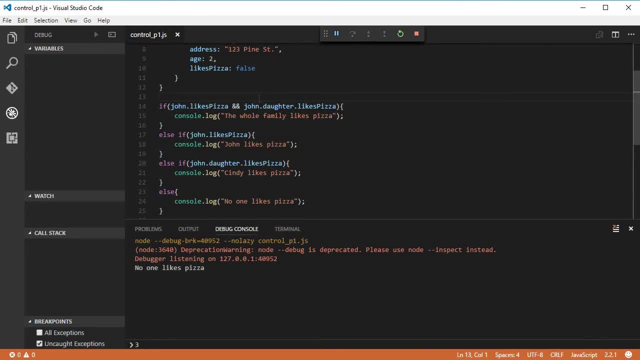 The logical operators we can go over are the and and ors, and or and not. So we're going to say, instead of John and his daughter, we can say John or his daughter likes pizza. In that case then it's going to say the whole family likes pizza. 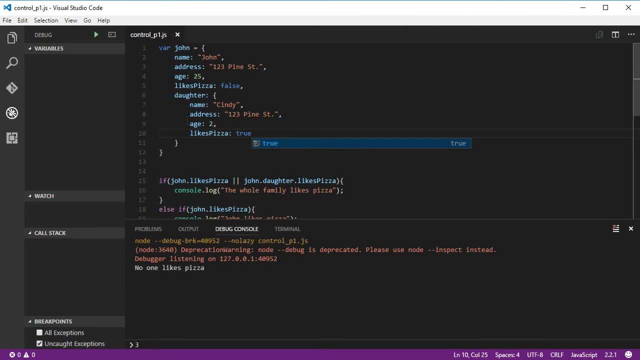 even though only one of them likes it. And in this case it's not ideal because we want to check for the whole family. But this is just showing, you know, or statement. The or statement says that he can either be true or she can be true. 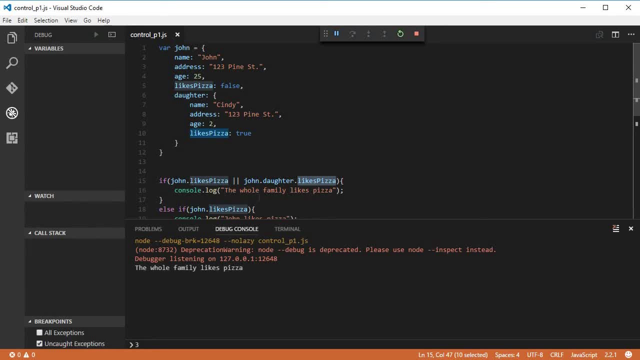 But one of them. as long as one of them is true, then this whole statement is fine. The next thing we're going to do an and again We're going to say: if John doesn't like pizza, we're going to negate that statement. 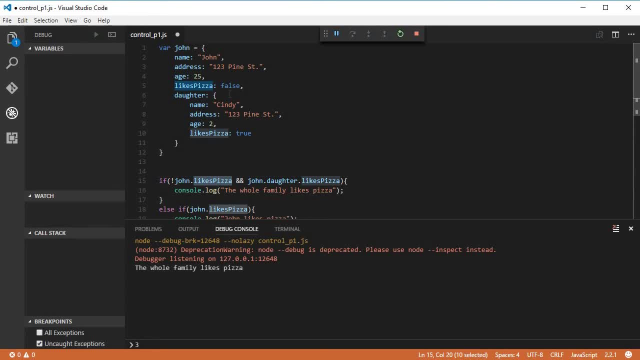 So what this is is showing whatever value he has right now. we're going to take the opposite value, which will be true. So in this case it'll say true and true, which then should say: the whole family likes pizza, Even though John is saying false. we're taking the opposite of what he says. 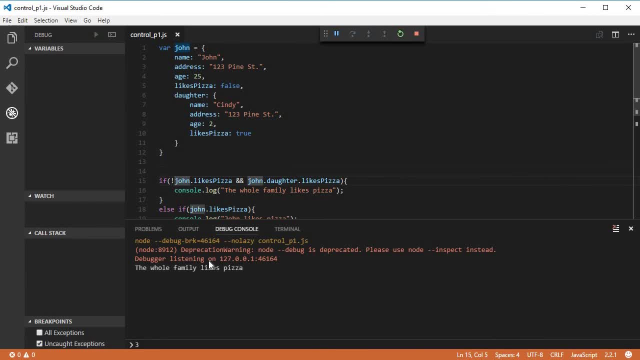 And sure enough we have. the whole family likes pizza. So that was a little bit on control statements and logic operators. The next video we're going to go over switch statements.